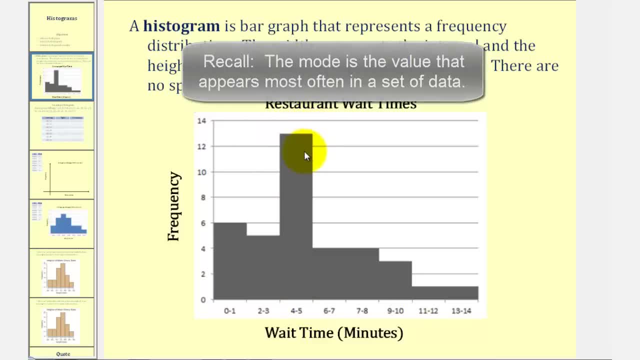 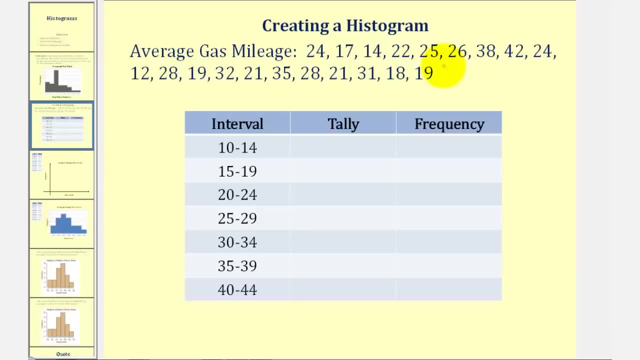 minutes, Looks like it occurred 13 times. Now let's construct our own histogram. Here we're given data on average gas mileage of 20 cars. So before we create the histogram, we'll complete this frequency table where we already set up the intervals. Once again, notice how they have the same width of the same 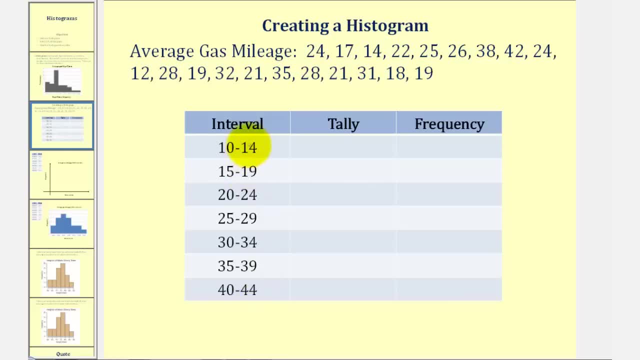 size and there are seven intervals. here We can say we have seven bins. So we'll first go through and tally the data in the correct interval and then find the frequency, So starting with 24, which would be in this interval. Then we have 17,, 14,, 22,, 25, and 26.. Both in this interval: 38,, 42,, 24,, 12,, 28,, 19,, 32,, 21,, 35,, 28,. 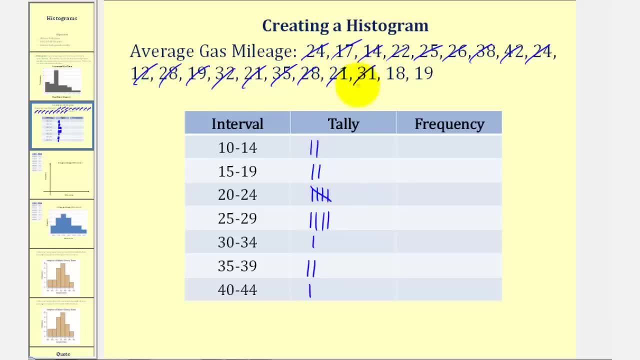 21,, 31,, 18, and 19.. And therefore the frequencies will be 2,, 4,, 5, 4,, 2,, 2, and 1.. So we'll use these intervals or these bins along the horizontal axis, and we'll use 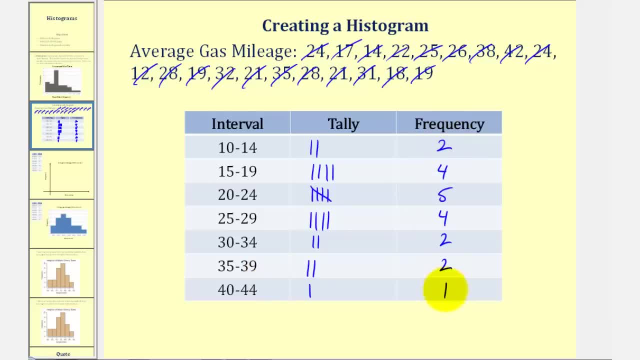 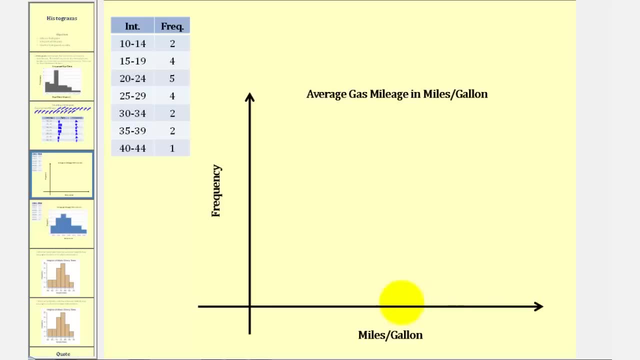 the frequencies along the vertical axis. Let's go ahead and set this up, Starting with the intervals of the bins. we'll divide the horizontal axis into seven equal intervals, So 1,, 2,, 3,, 4,, 5,, 6, and 7.. So let's go ahead and label. 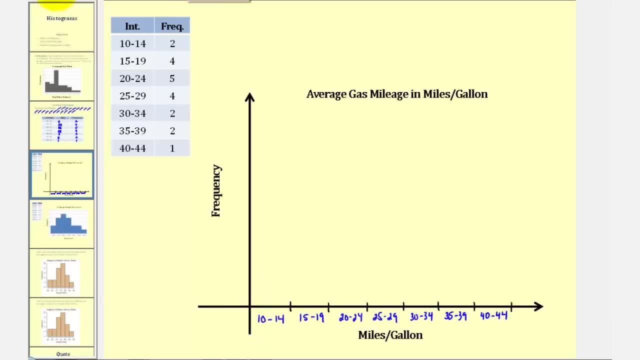 them, The highest frequency is 5.. Let's go ahead and have a maximum value here of 6.. Break this into 6 equal pieces, And now we'll construct a bar for each bin or each interval. So for the interval from 10 to 14, the frequency is 2.. So we make a bar with a. 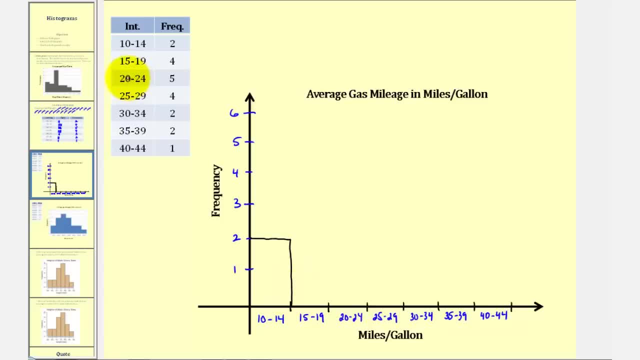 height of 2.. The interval from 15 to 19 has a frequency of 4.. So we make a bar with a height of 4 over this interval. The next interval has a frequency of 5.. So we make a bar of height 5.. 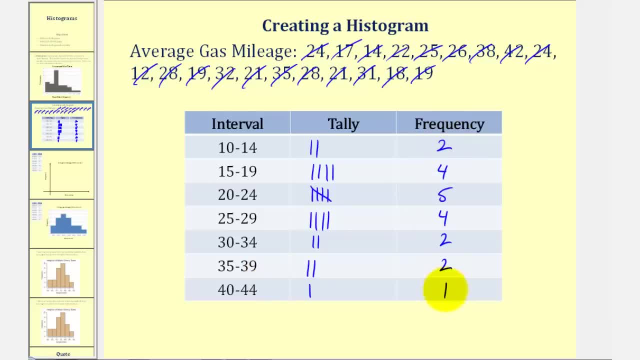 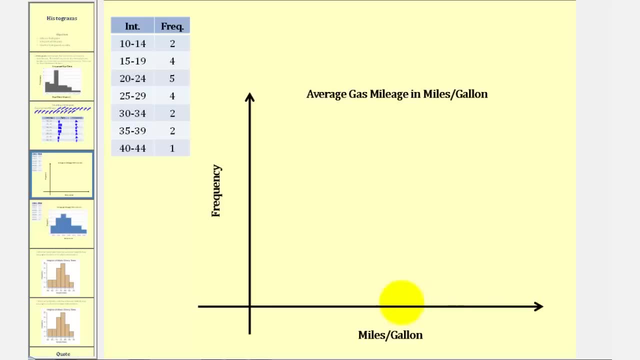 the frequencies along the vertical axis. Let's go ahead and set this up, Starting with the intervals of the bins. we'll divide the horizontal axis into seven equal intervals, So 1,, 2,, 3,, 4,, 5,, 6, and 7.. So let's go ahead and label. 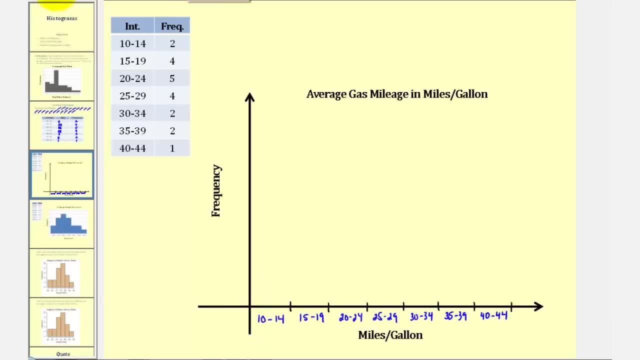 them, The highest frequency is 5.. Let's go ahead and have a maximum value here of 6.. Break this into 6 equal pieces, And now we'll construct a bar for each bin or each interval. So if the interval from 10 to 14,, the frequency is 2, so we make a bar with a. 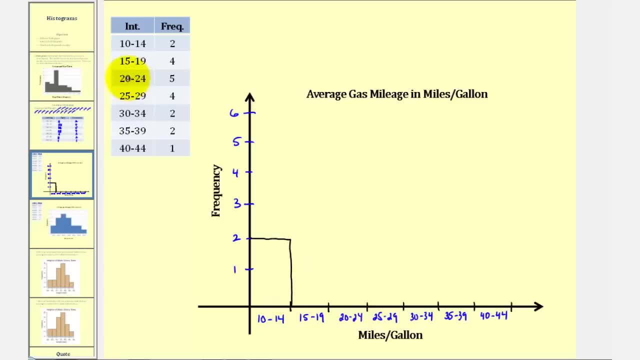 height of 2.. The interval from 15 to 19 has a frequency of 4, so we make a bar with a height of 4 over this interval. The next interval has a frequency of 5, so we make a bar of height 5.. 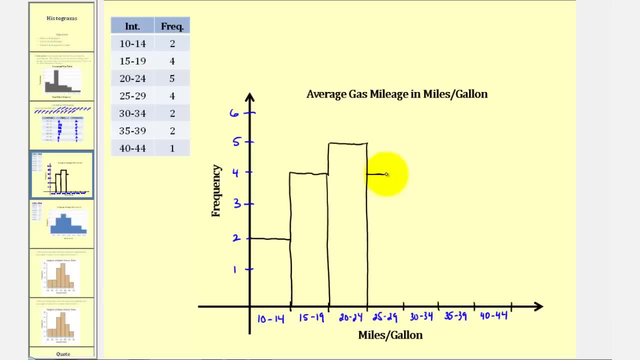 The next frequency is 4.. The next two frequencies are 2. And the last frequency is one. And here's our histogram And once again we can see that the mode would be the interval from 20 to 24 for this data of average gas mileage in miles per gallon. 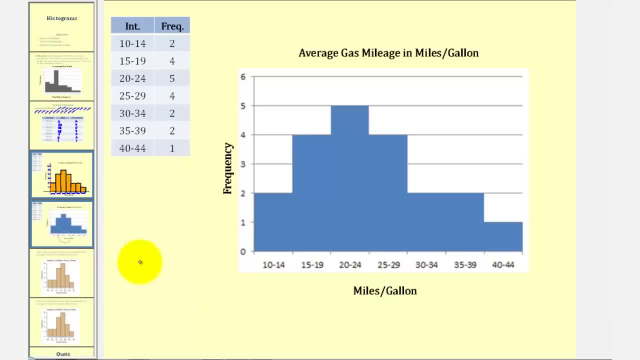 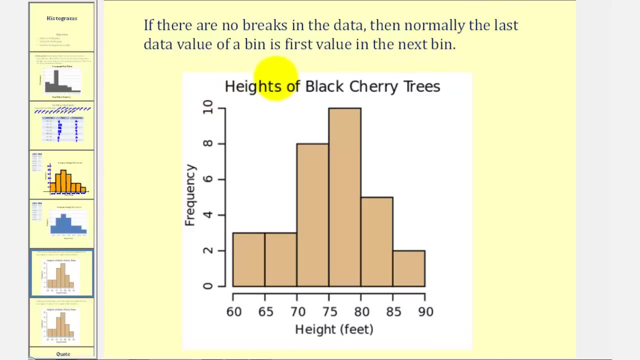 I went ahead and created this same histogram using some software, with the same results. This histogram was made with Excel. Here's one more thing I'd like to mention before we go. If there are no breaks in the data, then normally the last data value of a bin 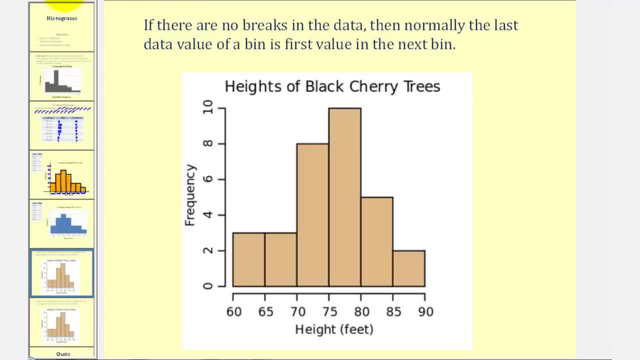 is the first value in the next bin. For example, looking at the given histogram on heights of black cherry trees, notice how the horizontal axis is labeled by fives. so this first interval, or first bin, looks like it goes from 60 to 65,. 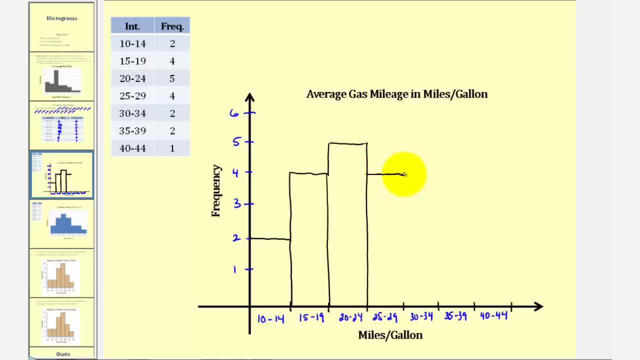 The next frequency is 4.. The next two frequencies are 2.. The next two frequencies are 2.. And the last frequency is one. And here's our histogram, And once again we can see that the mode would be the interval from 20 to 24. 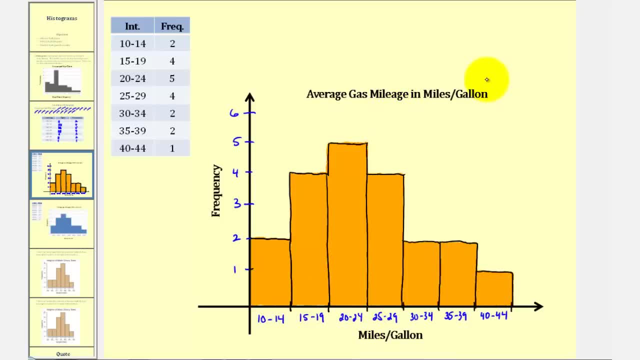 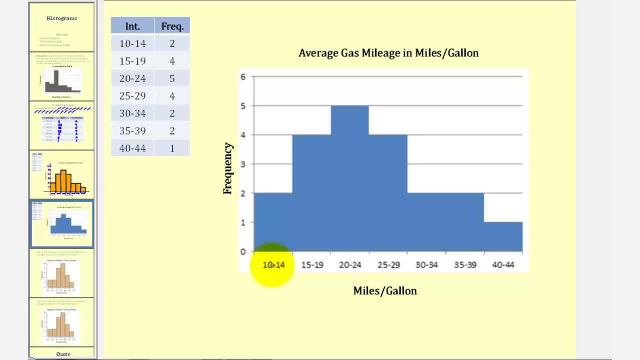 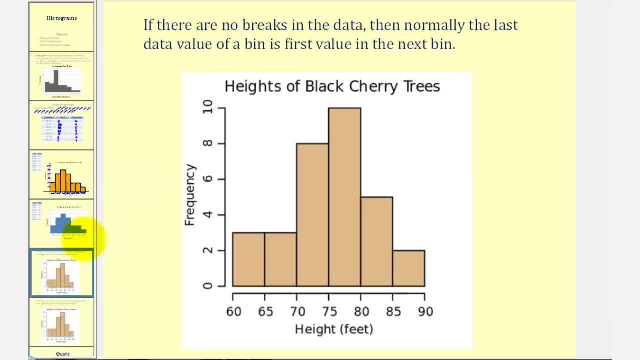 for this data of average gas mileage in miles per gallon. I went ahead and created this same histogram using some software, with the same results. This histogram was made with Excel. Here's one more thing I'd like to mention before we go, If there are no breaks in the data. 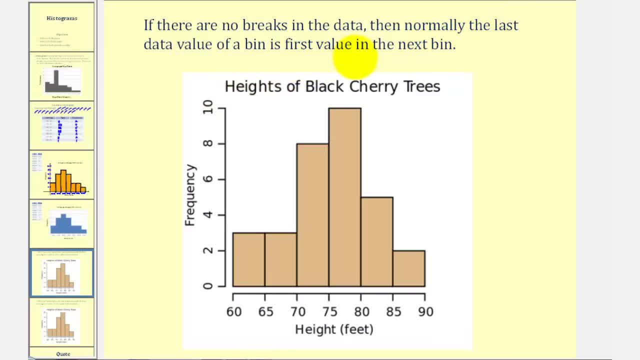 then normally the last data value of a bin is the first value in the next bin. For example, looking at the given histogram on heights of black cherry trees, notice how the horizontal axis is labeled by fives. so this first interval or first bin. 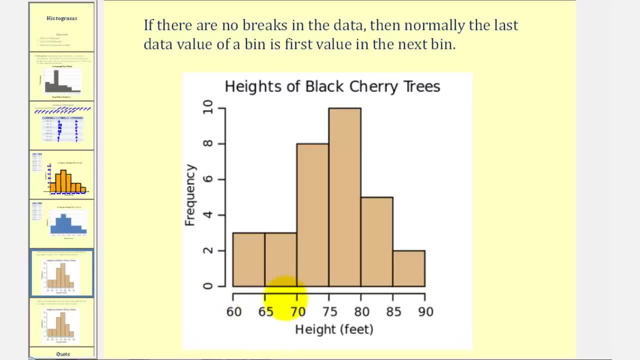 looks like it goes from 60 to 65, and the second bin, or second interval, goes from 65 to 70. So the question becomes: where is the 65? Is it in the first bin or is it in the second bin? 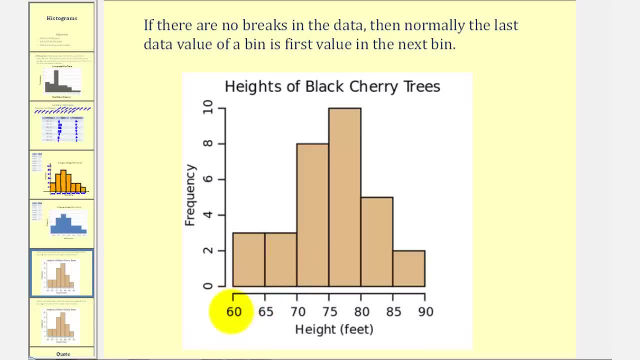 And it's actually in the second bin. This first interval is from 60 to 65, where, if we use interval notation, it would be closed on 60, meaning it includes 60, but it would be open on 65, meaning it does not include 65.. 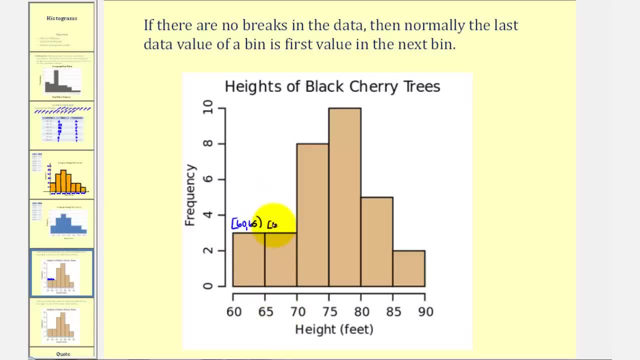 The next interval would be closed on 65 and open on 70,. the value of 70, would be in this third interval. The third interval would be closed on 70,, meaning it includes 70,, but open on 75,, meaning it does not include 75, and so on. 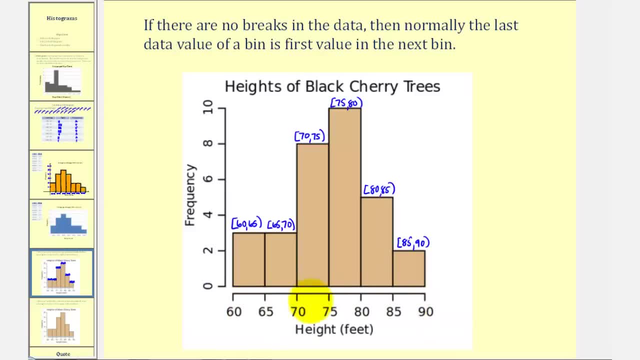 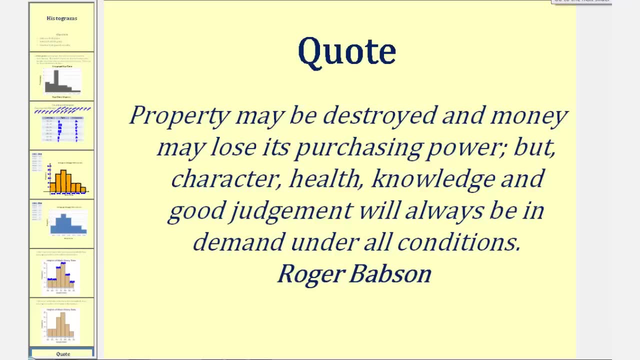 So it is important to keep this in mind if you see a histogram labeled, as we do here. I hope you found this helpful. Thank you.